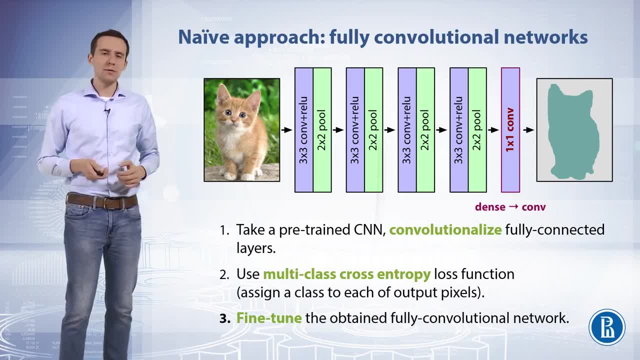 field one by one. When we do this, we gain some form of localization if we look at where we have more activation. The optional step is to fine-tune the fully convolutional network for solving the segmentation task. Important point to note here is that the loss function we use in this image segmentation. 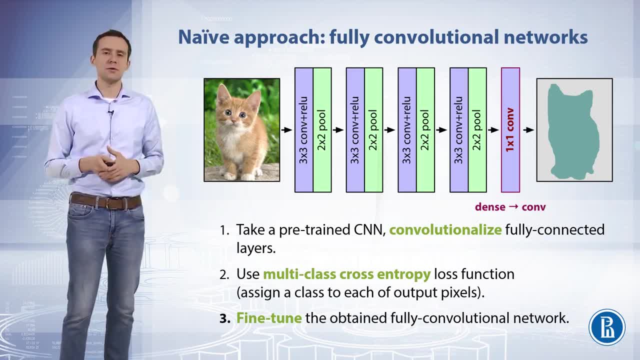 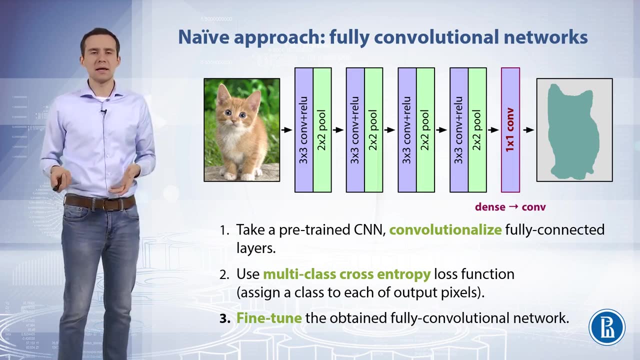 scenario is actually still the usual loss function we use for classification- Multi-class Loss entropy, And not something like the L2 loss like we would normally use when the output is an image. This is because, despite what you might think, we're actually just assigning a class to each. 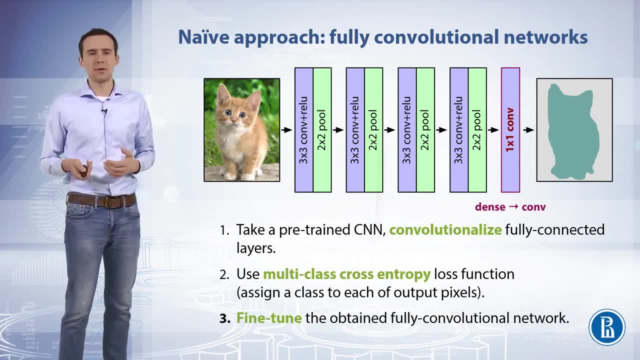 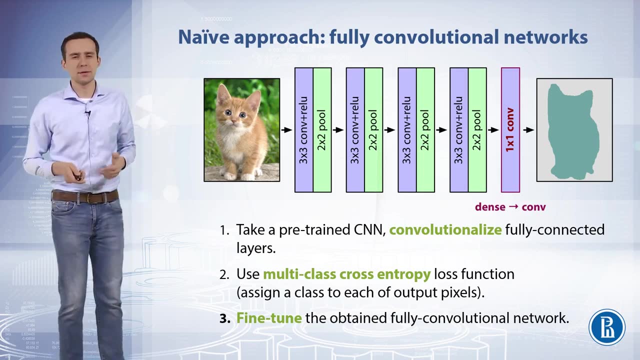 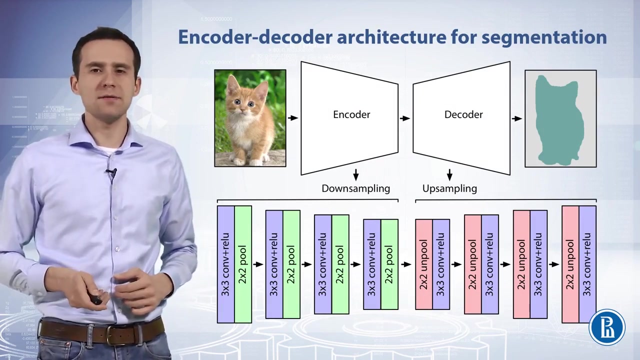 of our output pixels. So this is a classification problem. The problem with this approach is that we lose some resolution by just doing this, because the activation were downscaled on a lot of steps. Example with: the cyclist is on the slide. Different approach to solving semantic segmentation via deep learning is based on downsampling-upsampling. 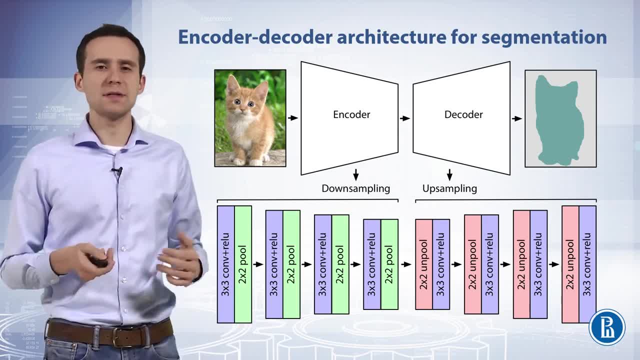 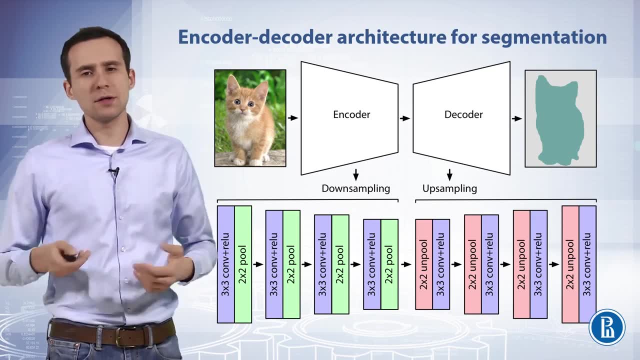 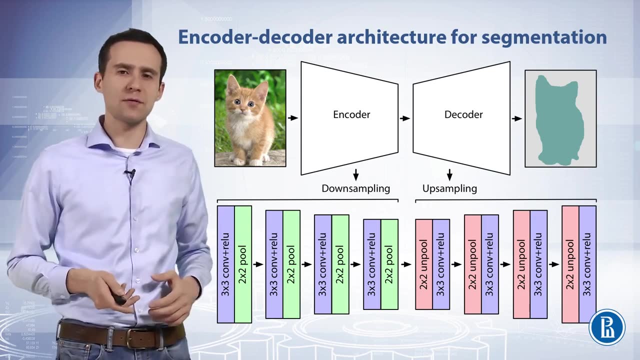 architecture where both left and right parts have the same size in terms of number of trainable parameters. This approach is also called the encoder-decoder architecture. The main idea is to get the input image with size n times n, compress it with a sequence of convolutions. 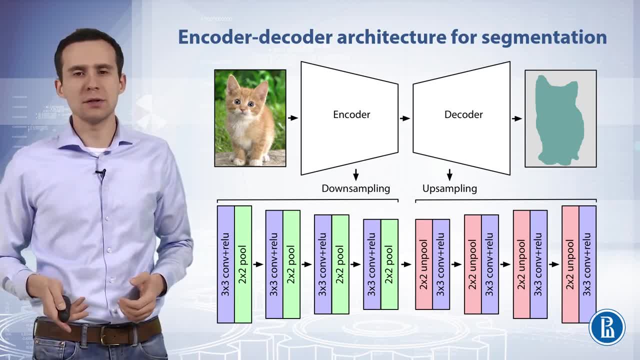 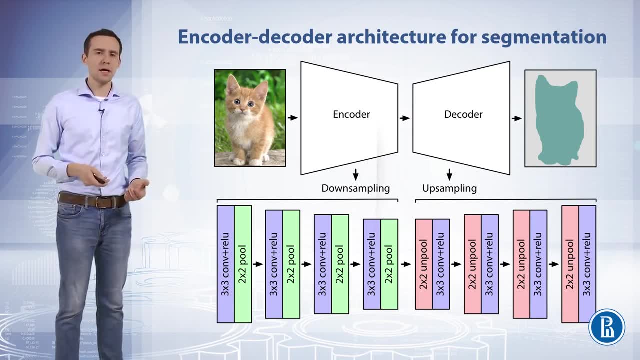 And then decompress it And get the output with the original size n times n. How can we do that? To save the information we could use skip connections or reserve all convolution and pooling layers by applying unpooling and transpose convolution operations in deconvpart, but at 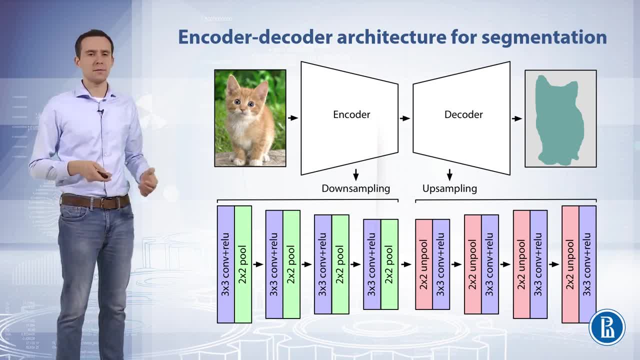 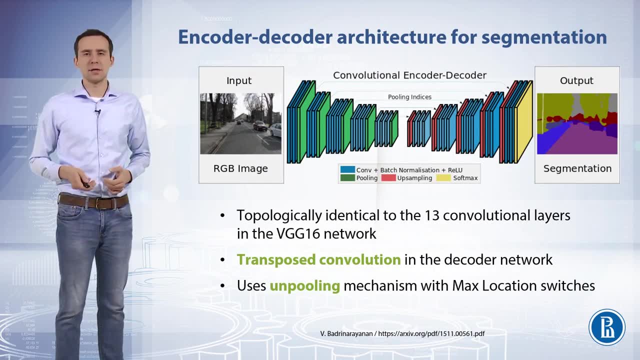 the same place as where maxpooling and convolution is applied on convolutional part or encoder part of the network. A working example of such an architecture is this: This is the SEGNET model featuring a VGG identical encoder or downsampling part and the corresponding 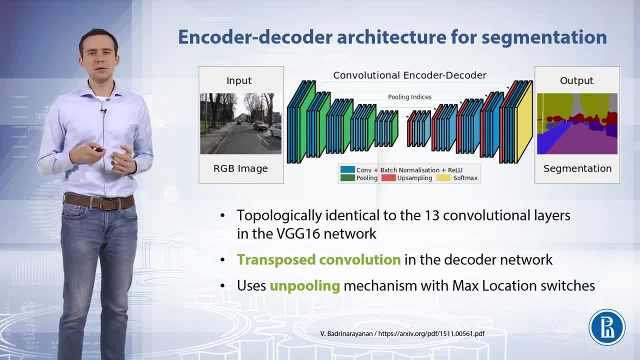 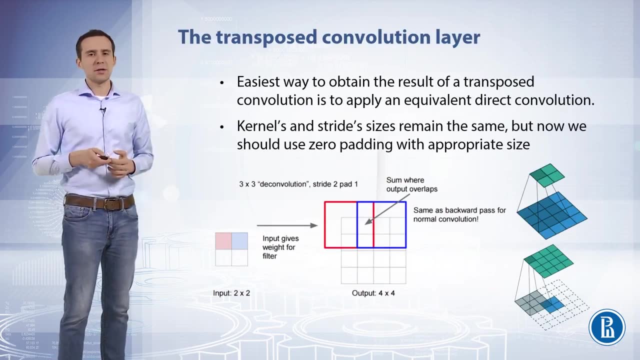 decoder or upsampling part. While possessing many learnable parameters, the model performed well for road scenes classification on the CAM-VID dataset, while slightly underperforming for segmentation of medical images. Let's look at the details of transposed convolution employed in the SEGNET model. 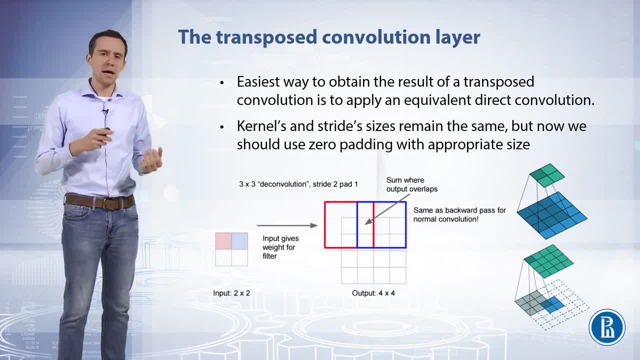 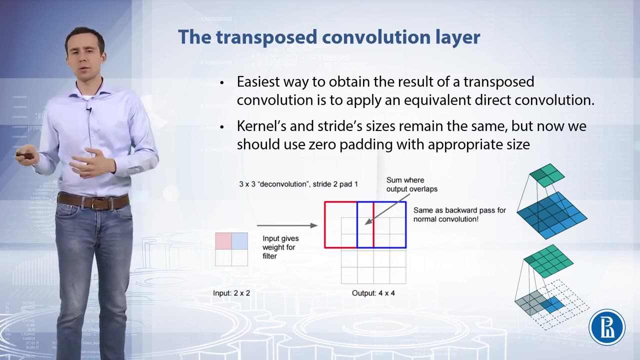 Basically, The idea is to scale up the scale down effect made on all previous layers. Actually, the upsampling forward propagation is the convolution back propagation and the upsampling back propagation is the convolution forward propagation. The easiest way to obtain the result of a transposed convolution is to apply an equivalent. 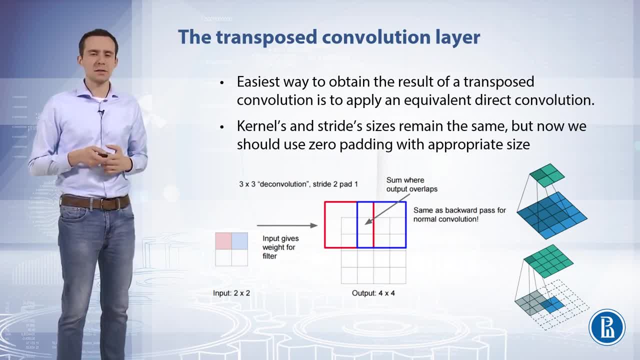 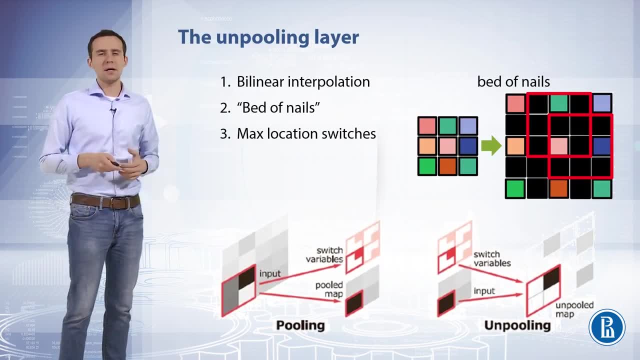 direct convolution. Kernel and stride sizes remain the same, But now we should use zero padding with appropriate size. For better understanding of downsampling-upsampling architecture, we need to study the mechanism of unpooling. The maxpooling operation is non-invertible. therefore one may consider different approximation. 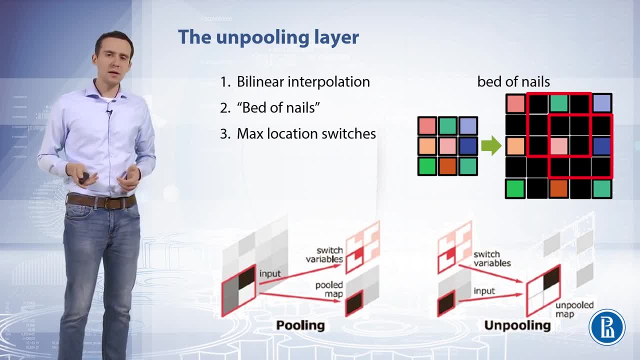 to the inverse of maxpooling. The easiest way is to use resampling and interpolation. This means taking an input image, rescaling it to the desired size And then calculating the pixel values at each point using an interpolation method such as bilinear interpolation. 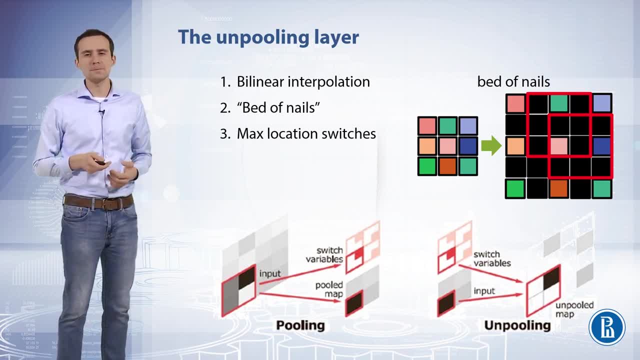 Another idea to restore maxpooling is a bed of nails where we either duplicate or fill the empty block with the entry value in the top left corner and zeros elsewhere. Yet another ineffective mechanism is the following: We record the position called maxlocation switches, where we located the biggest values during. 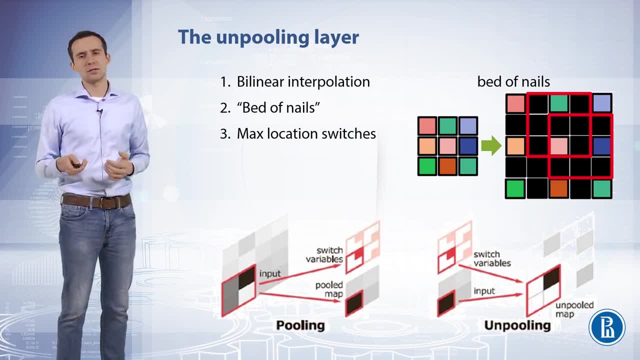 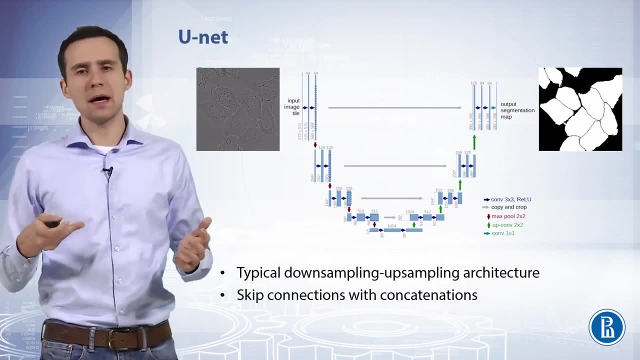 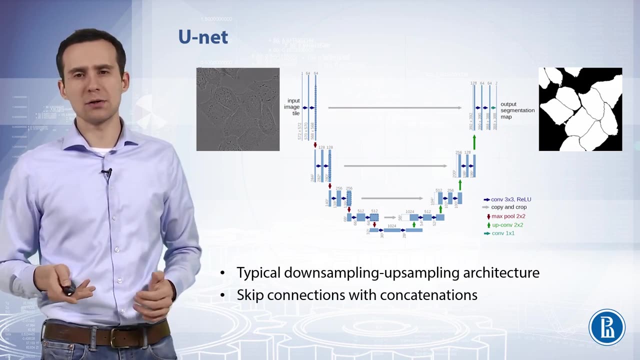 normal maxpooling and then use the positions to reconstruct the data from the layer above U-Net. yet another model is a downsampling-upsampling architecture, illustrated on the slide. The downsampling part follows the typical architecture of a convolutional network. 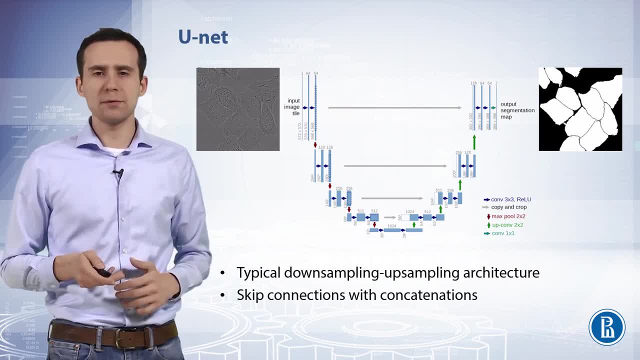 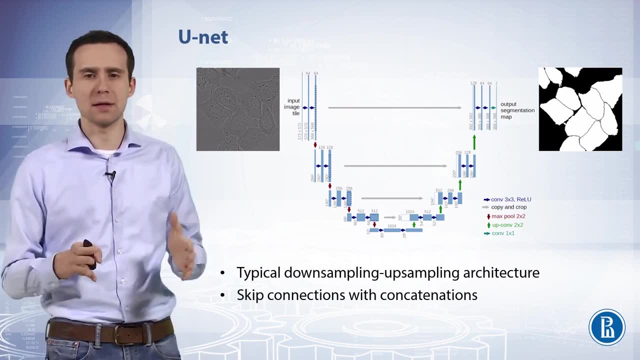 It consists of the repeated application of two 3x3 unpadded convolutions, followed by a rectifier linear unit and a 2x2 maxpool in operation with stride 2 for downsampling. At each downsampling step, we double the number of feature channels. 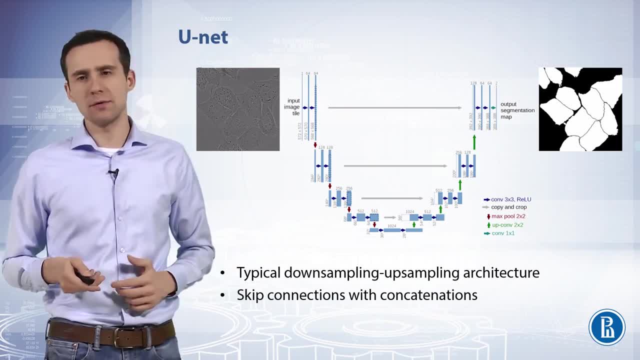 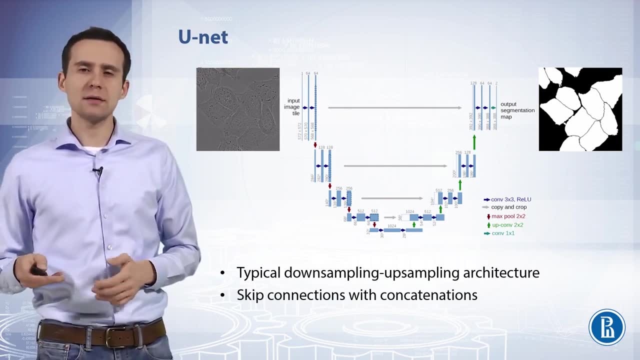 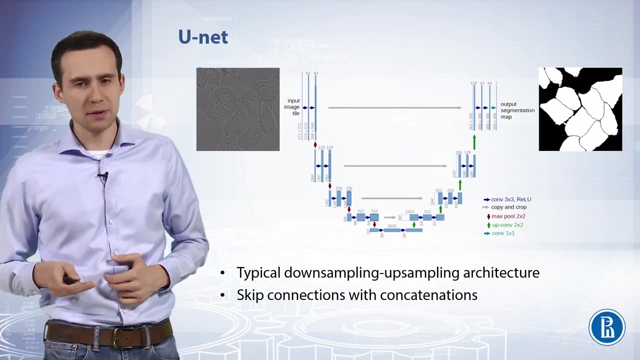 Every step in the upsampling part consists of a transposed convolution of the feature map, followed by a 2x2 convolution that halves the number of feature channels and upsamples the data, and a concatenation with the correspondingly cropped feature map from the downsampling.